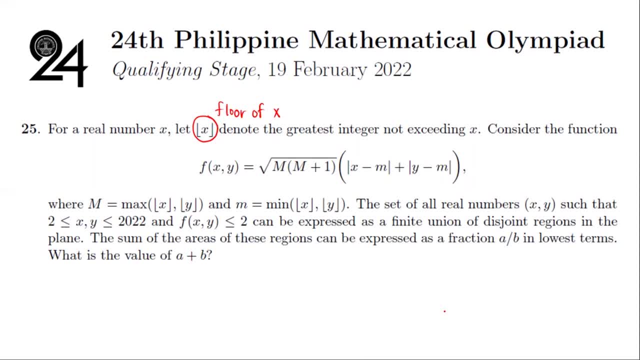 floor of x and y, and small m is the minimum of the floor of x and y. Well, that means that I already did this. So, anyway, he, him me, and that of the man, me and The set. 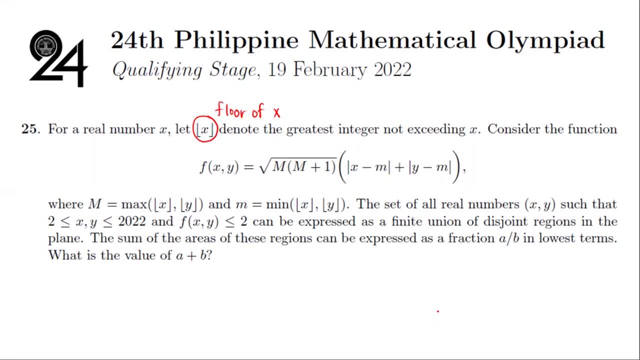 of all real numbers, x, y, such that x and y are between 2 and 20,, 20,, 2.. And f of x, Y is less than or equal to two, can be expressed as a finite union of this joint regions in the plane. The sum of the areas of these regions can be expressed: 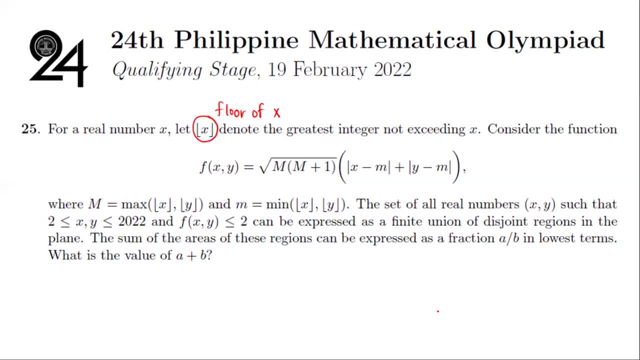 as a fraction: a over b. in lowest terms, What's the value of a plus b? So the PML qualifying stage is a contest where it's convenient to have a single number as the final answer, and it's going to be for it to be an integer. So that's why the problem was formulated as: 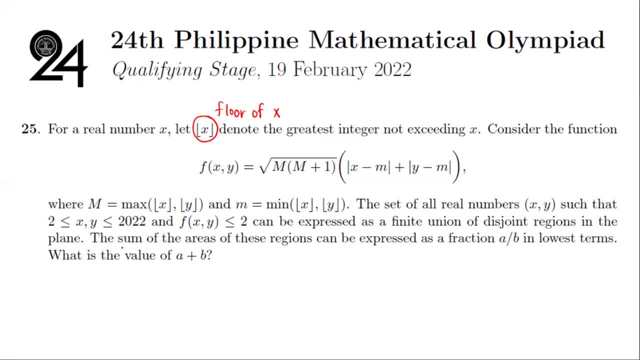 finding the value of a plus b, but really it's the some of the areas that we're interested in, so we're going to be focusing on figuring out what this fraction a over b is. now the problem is talking about certain regions of which we have to find the area. so these are the collection of points x, y. 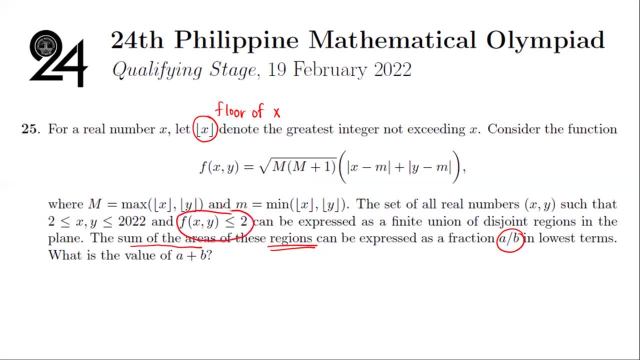 for which the function's value becomes less than or equal to two. so i suppose for different values of x and y the output could be larger than two. sometimes it's going to be less than or equal to two, but apparently if we want that inequality to hold, that's going to happen when x and y somehow. 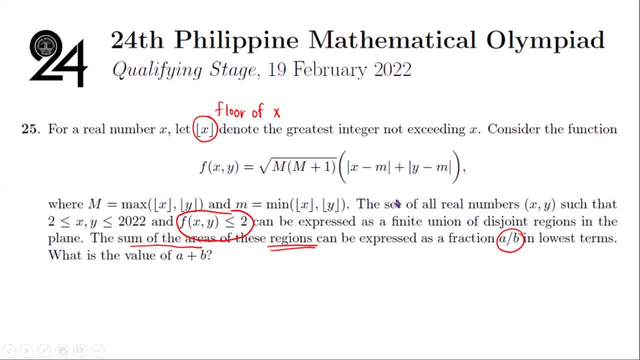 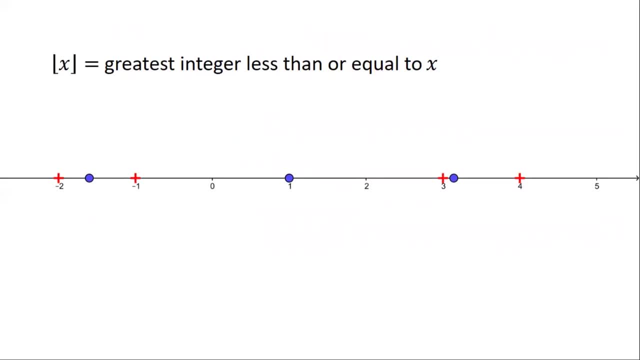 belong to certain regions, so we want to understand how those regions are going to look like. but first let's have a look at the floor function. so f of x, sometimes denoted by this notation or this notation which the problem uses. so this is the greatest integer function. 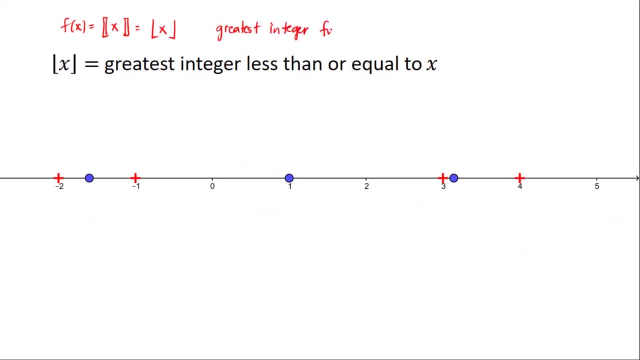 greatest integer function, sometimes also referred to as the floor function. for those who want to know more about this function, you can refer to videos number eight and nine in the current uh tutorial series that we have here for the philippine math olympiad. so this is the greatest integer less than or equal to x. here are some examples: pi is a number. 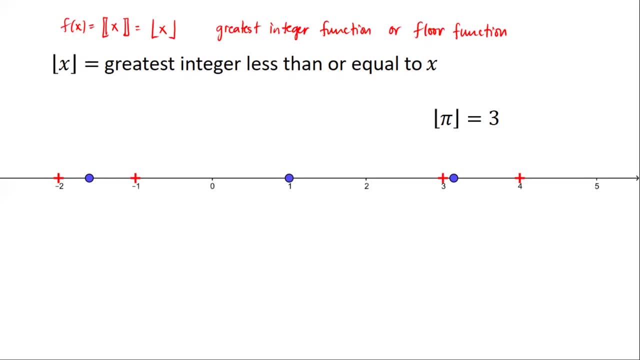 between three and four, because it's approximately 3.14. so three is the greatest integer, just before pi. so what this suggests is to find the floor of x we round down. so it's not really rounding off because even if it was 3.9, which is closer to four, three is still the greatest integer. 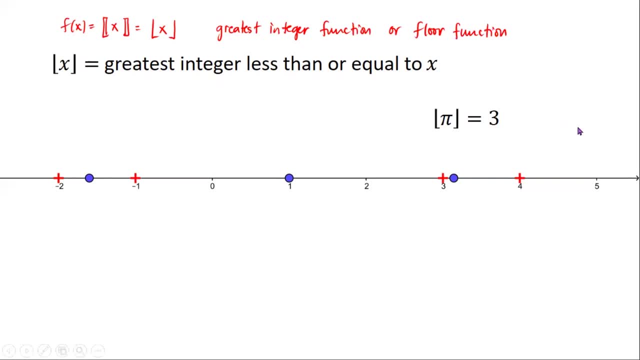 just before three, sorry, just before pi, and then uh, for negative 1.6, which is between negative two and negative one. so the floor of that is negative two. but what if the integer is cx? so for example, the floor of one is equal to itself one, because hey, it's already an integer, so there's no need to. 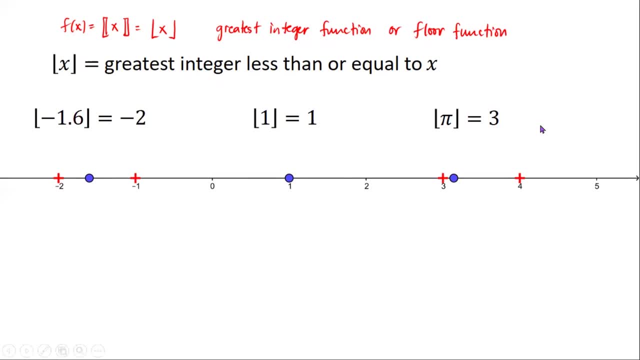 um, there's no need to round down now some of the properties that we're going to need. so if x is greater than equal to n, but strictly less than n plus one, so in other words, uh, let's say x is one of those points in the blue segment starting from n up to just before n plus one. 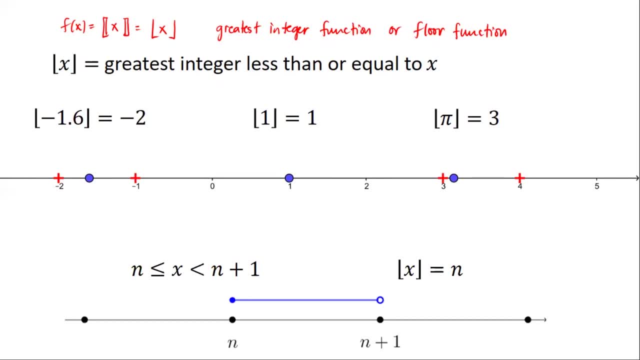 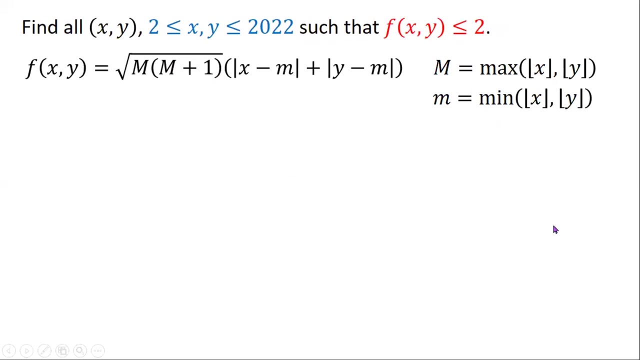 where n is an integer here. so for all these points, their floor is equal to n. so x equal to n plus one is in excluded, because in that case the floor of x would jump and become n plus one. okay, so let's go back to the problem. so there's a lot happening here, so there's a lot of different parts. 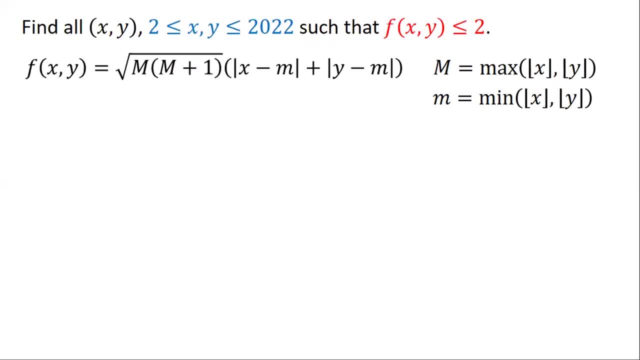 and pieces, there's a uh, there's this big m and small, and where you have to choose between the floor and the, between the maximum and the minimum of the floor. now, um, so, sometimes when you look at the solution to a problem from step one to step two, to step three, but sometimes solutions do not show the process that 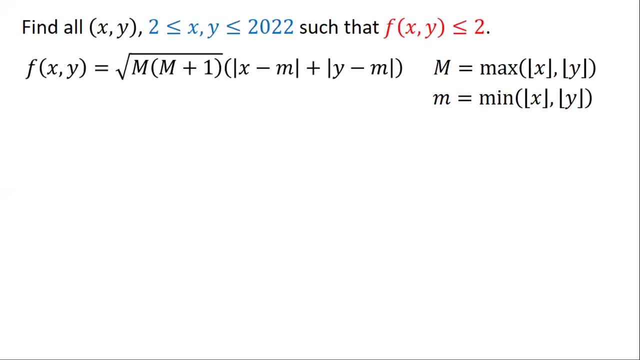 it took to arrive at that solution, and sometimes it's messy as you try to make sense, and the button function f, but one thing's for sure: we need to be able to understand this, and sometimes what helps is to consider, uh, special cases. so when I attempted this problem, 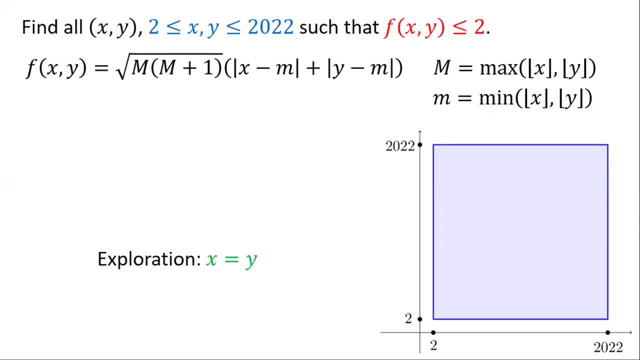 I started by assuming. suppose x is equal to y. now the square there on the right consists of all the points x, y, such that the coordinates x, y are between 2 and 2022.. so this is not drawn to scale, but I think it's enough to, uh, give us an idea. 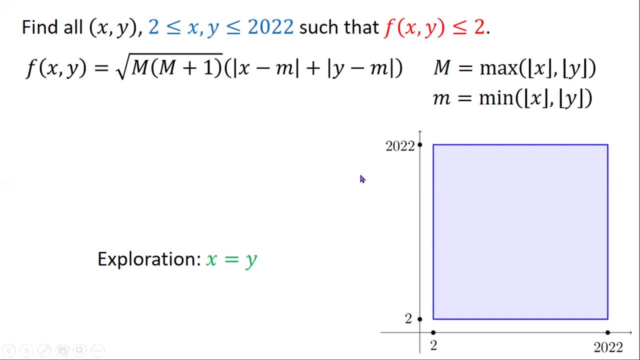 now, all the points for which x is equal to y are therefore going to be all the points on the line bisecting the first quadrant. so that would be that green diagonal inside the blue square. so points x, y on that green diagonal, such that f of x, y is less than or equal to the number two. 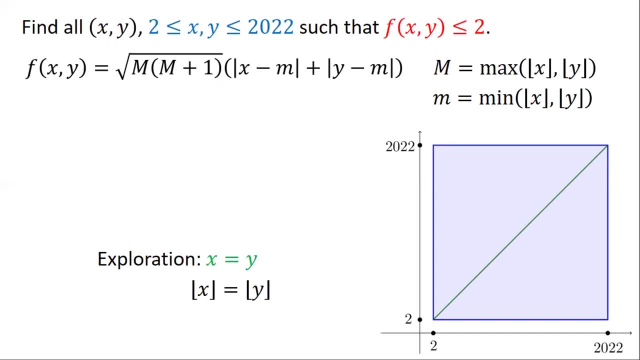 now, because x is equal to y, then their floor functions are the same, and let's give that a name for the common value, small n, and therefore for the maximum and minimum, big M and small M. we don't really have to make a choice. fortunately, small n, and so we can. 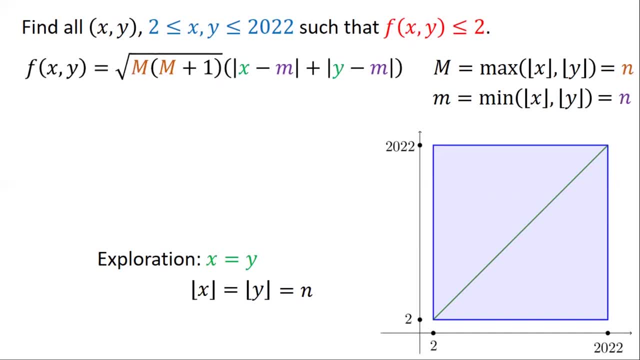 incorporate that into the function and note that x and y are equal. so when we make the replacements, this is what we get now: the two absolute value expressions are equal. so you can write that doubled. and furthermore, because n is the floor of x, n is the result of rounding down. X is greater than or. 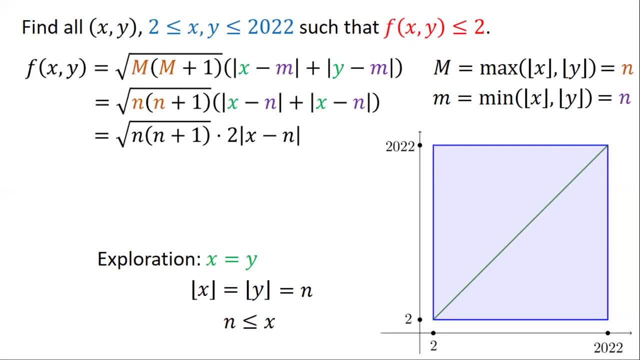 to n. so by the relationship 3.14 or pi is greater than or equal to 3. so you can drop the absolute value bars, so it's just twice x minus n. so we are looking at the following situation: we want this to be less than or equal to 2, or you can cancel the twos from both sides of the, from both sides of. 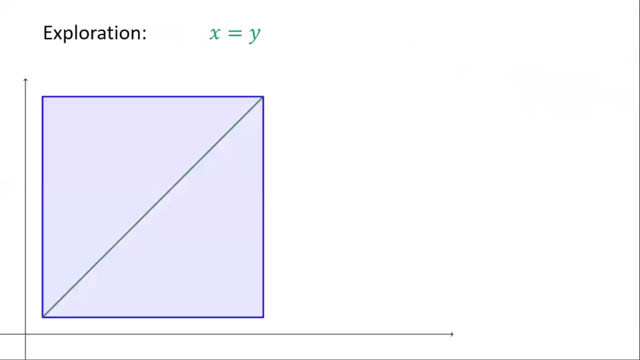 the inequality. so you get this and uh, so we have more space because we're running out, okay, so again, we were assuming x is equal to y and the floor is equal to n for them. so this is the inequality that we ended up having, which means x is uh. well, because x is between n and n plus 1, so i marked. 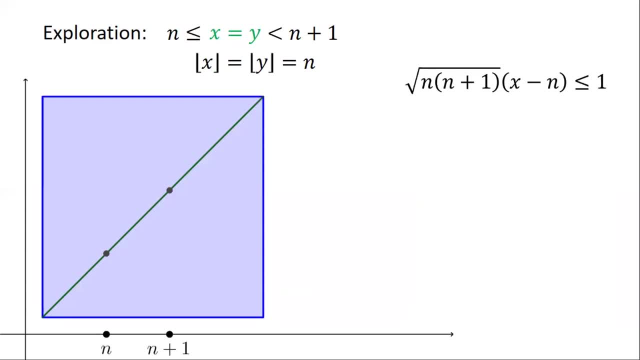 them on the x axis and then the points we're looking at are on the green diagonal, so they must be from within that segment between those two grayish points. but in particular, because of this inequality, we also want x to be less or equal to n, so something over n plus what this fraction 1 over n times. 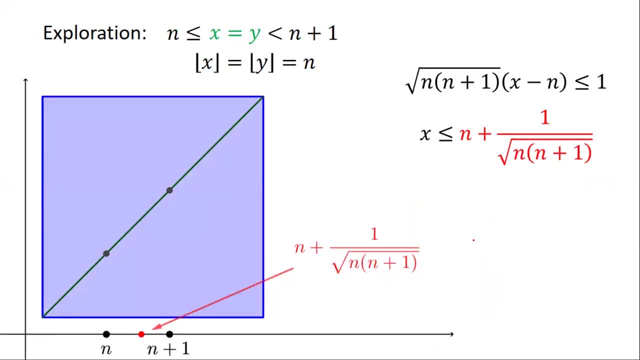 n plus 1.. now, uh, that's going to be there, between n and n plus 1.. so observe that this fraction, this is not going to exceed 1.. so we're sure that that red point is definitely between n and n plus 1.. so if the x coordinates have to satisfy that inequality, then that means the 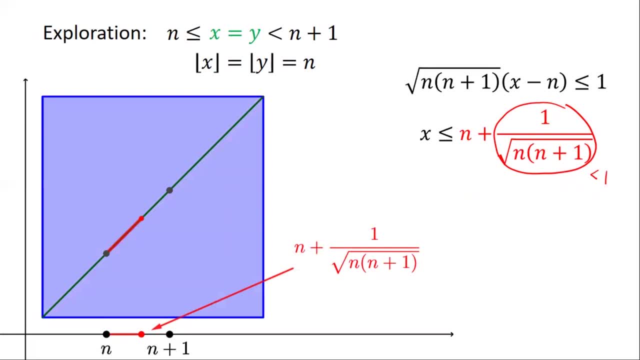 points that we are looking at between n and n plus 1 on the x-axis. that would have to be the points on that particular red segment. okay, but back to the problem. so at the start i was wondering the different regions we're looking at, are they going to be? 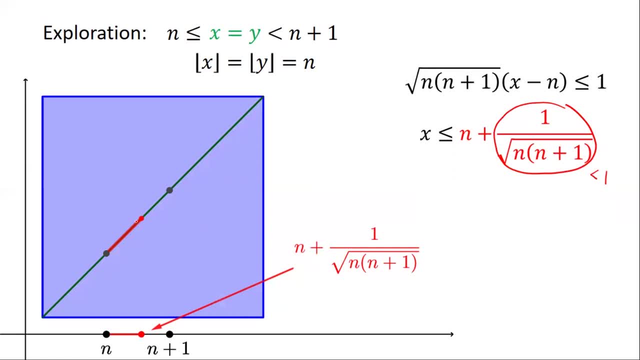 well, definitely they're going to include, uh, the many different red segments like that. so i was thinking, is it going to be a square like that, or is it going to be a horizontal and vertical strip? so, uh, it was all part of hypothesizing and looking at long money, but anyway, in the end we're going to 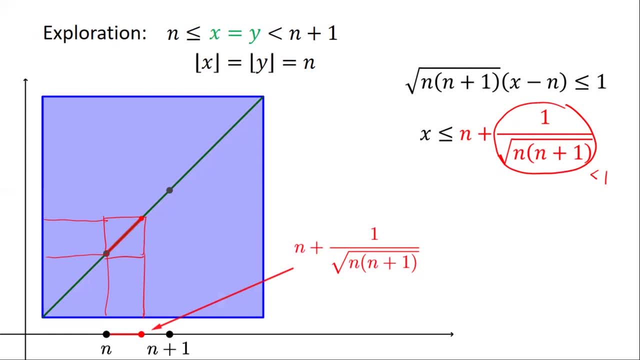 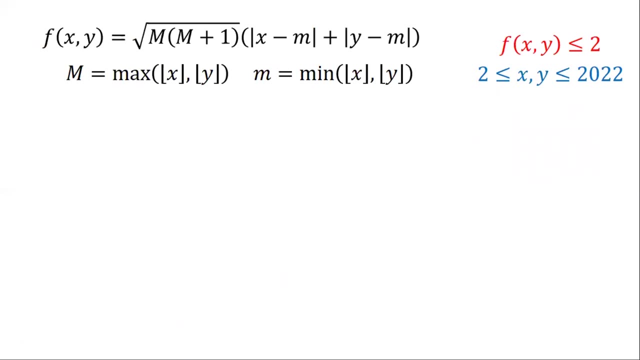 see that none of these regions will turn out to be the right region. all right, so let's continue, okay. so earlier i benefited from the assumption that x and y are equal, because then the floors of x and y are the same, so maximum and minimum, say, compare. 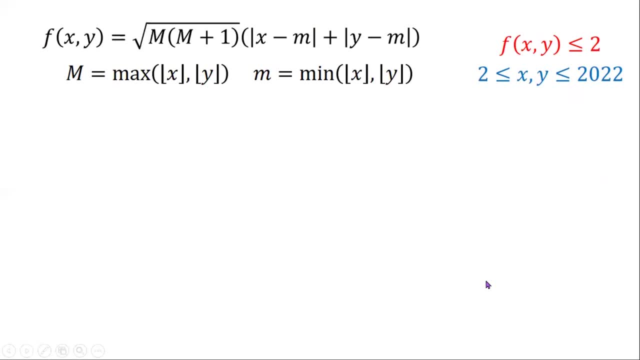 but So I thought, what if kailangan mamili? Let's say the floors of X and Y are different. So let's say Y is less or equal to X. So mas nasa kaliwa si Y, nasa kanan si X. 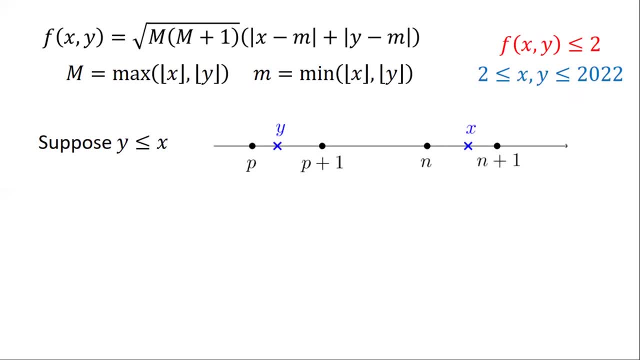 And suppose furthermore that they belong to these two different intervals. Y is in P to P, plus one somewhere on the left. X is somewhere on the right between N and N, plus one where P and N are integers. So that means the floor of Y is equal to P. 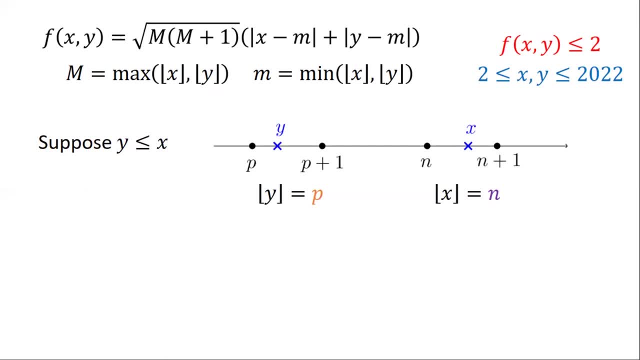 And the floor of X is equal to N. So we can see that P is smaller and is larger. So when we choose big M and small M, they're going to be small N- the larger one, and small P, the smaller one, respectively. 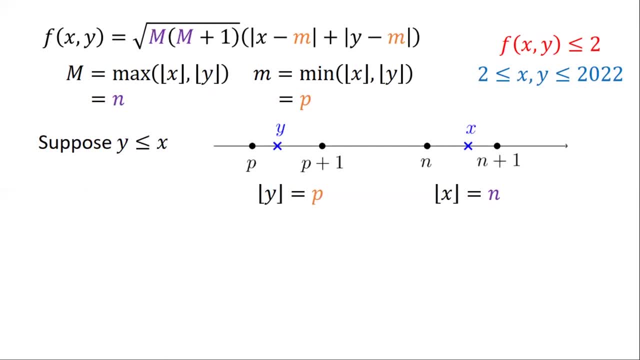 So we can make the replacement on the function F. So yeah, the square root of N, N plus one, And then the sum of those two absolute values where we replace small M by P, And, because of what we saw earlier, how we were able to actually drop the absolute value bars. 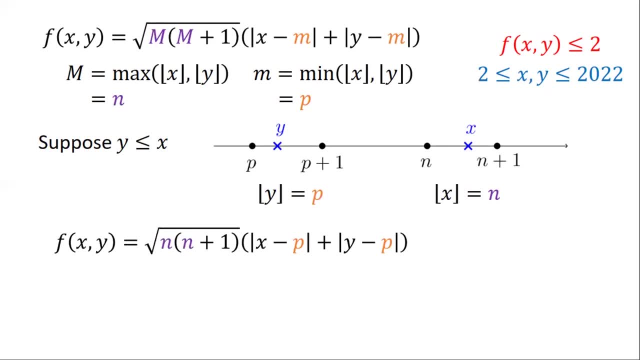 if you look at the drawing there, we can see that X is bigger than P and Y is bigger than P. So the absolute value expressions, we can replace them, as they are just X minus P and Y minus P. So here's the thing. 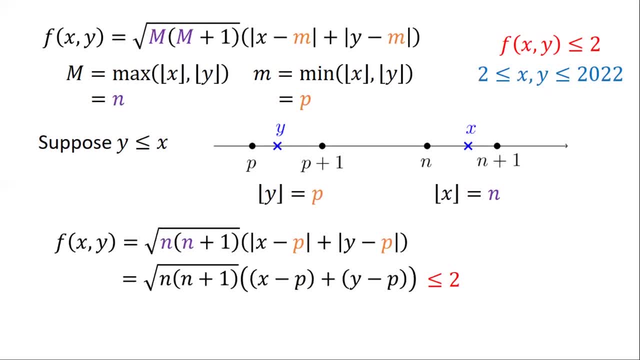 So we want this expression to be less than or equal to two, So that it evokes this idea that this expression should be small. Now the values of X and Y. so they start off small but they can be as large as 1,000,, 1,500,. 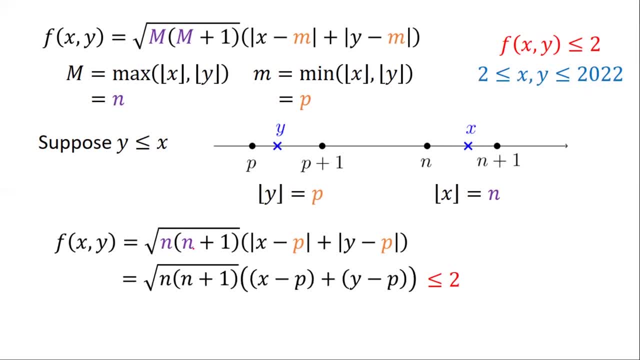 or not more than 2,022.. So that led me to thinking of how this first factor is going to be large And yet we want this, this product, to be small. So if the first factor is large, their product can still be small. 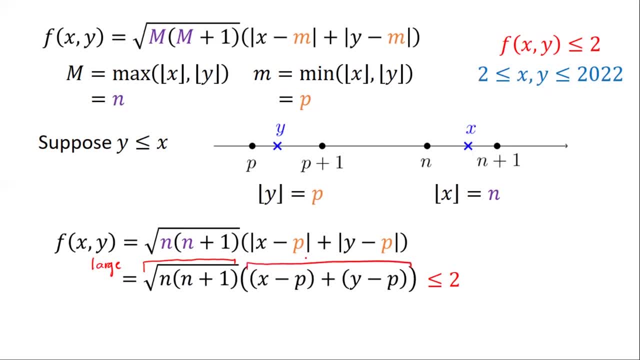 so long as we guarantee that the second factor is going to be small. It can't be as large as 2,022, otherwise it will exceed 2,022.. All right, Now, if you look at the square root of N times N plus 1,. 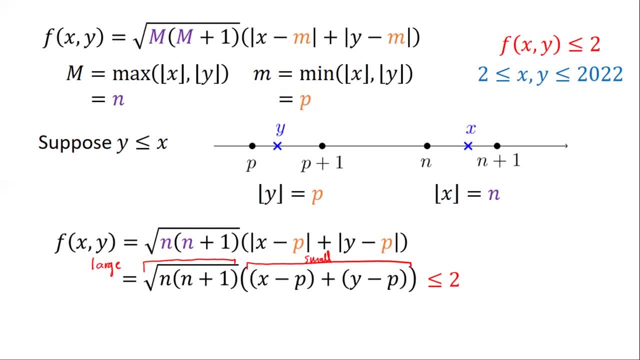 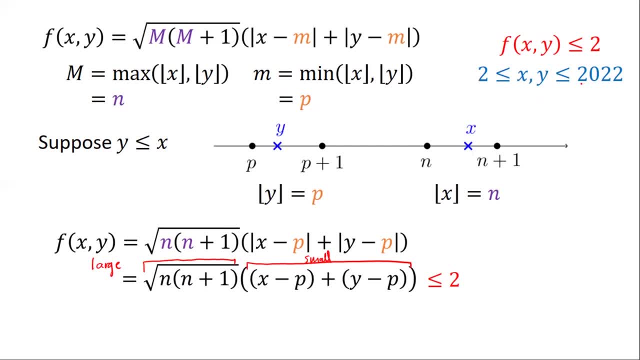 So they're between 2 and 2,022.. So well, the year now is 2022.. So that suggests to me personally, but I was wondering how, up to this point, we haven't used yet the lower bound. Why? 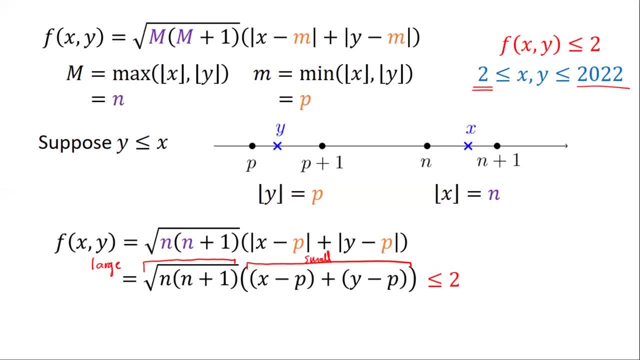 2? Why Can it be 3?? Or can it be 1?? All right, Well, because x and y, they're both greater than or equal to 2.. And n is the result of rounding down to the integer just below x. So that suggested. 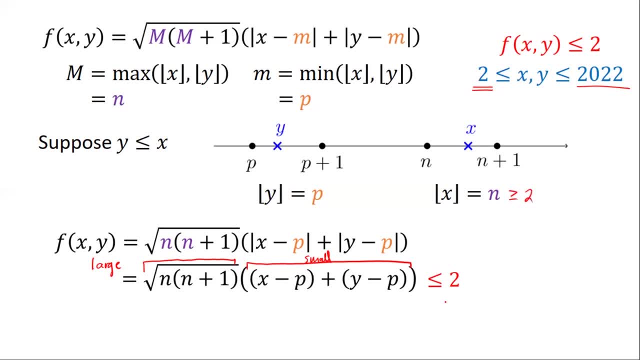 to me that n is greater than or equal to 2.. So even if you try to figure out the smallest value of the first factor, the one with n, n plus 1. So we see that this is going to be larger than the square root of 2 times 3.. So square root of 6, it's not a perfect square, But that's larger. 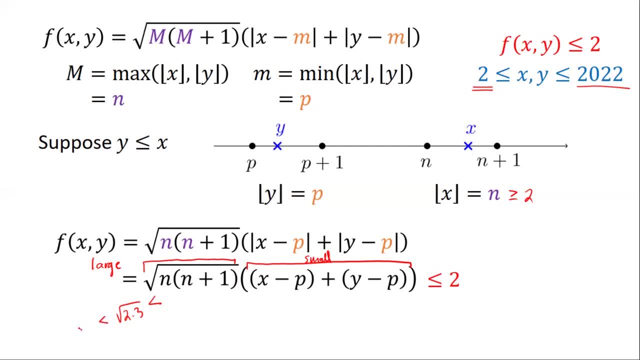 than the square root of 4.. That's a perfect square, which is 2.. So we see that the first factor, it's not even going to be equal to 2.. All right, The first factor, and it's being large, it's greater than strictly larger than 2.. And yet, 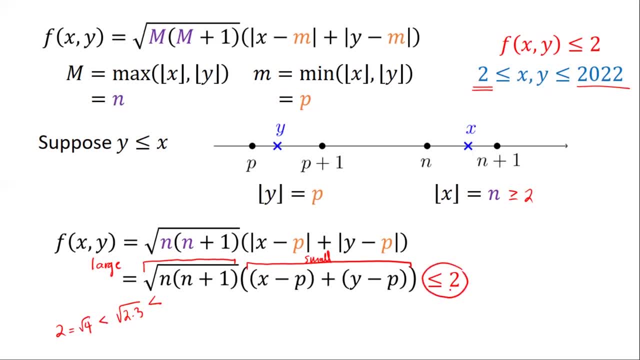 we want the product to be less than or equal to 2.. So, therefore, the only way for this condition- for the product to be less than or equal to 2, the only way for that to happen is that the second factor, this must be smaller than 1.. Okay, This must be smaller. 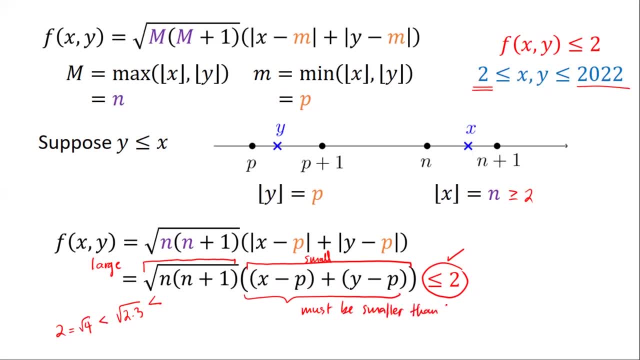 than 1.. All right, Because even if it's equal to 1,, if you multiply that to the first factor, it's already strictly larger than 2.. So the product would therefore be strictly larger than 2.. But it should be less than or equal to 2.. Okay Now, when I went back to look at the figure, 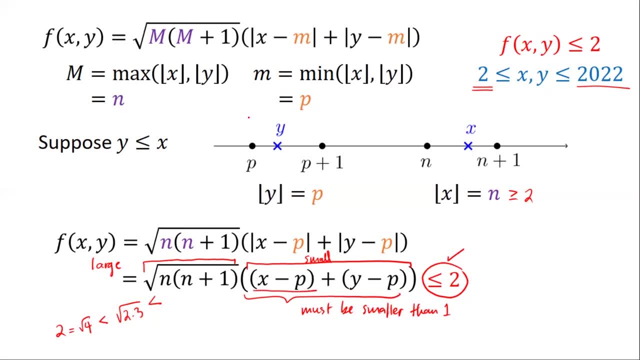 observe that the first term here, x minus p, measures the distance between the first and the second factor. So the first term here, x minus p, measures the distance between these two points, x minus p. And this is where I noticed that 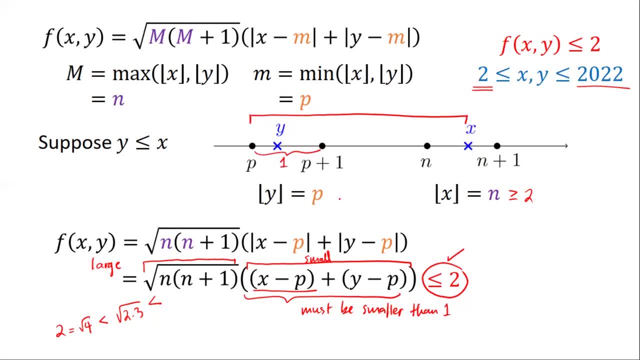 from p to p plus 1, that's already a distance of 1.. So, okay, it's possible that x is there at p plus 1, or x is just immediately after p plus 1.. But what this illustration showed me is that 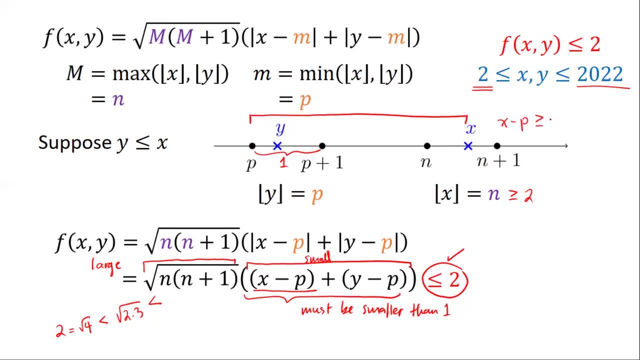 if you look at the difference of x minus p, that's already greater than or equal to 1.. So, therefore, if you look at this particular sum- okay, this particular sum- because of x minus p, this is already going to be greater than or equal. 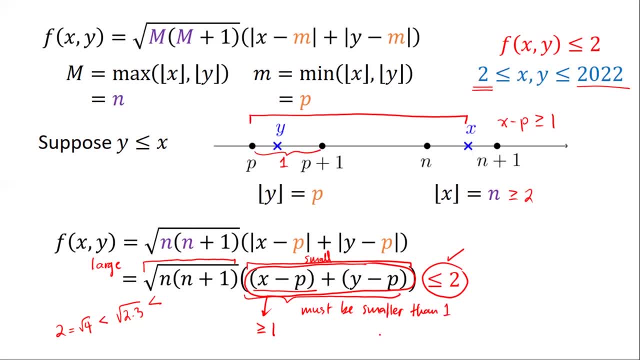 to 1, even if y minus p is 0. And we said that this sum must be strictly smaller than 1.. Which means this cannot happen. It's impossible for this second factor to be strictly smaller than 1.. Which means- this is our dream- that when the function of x minus p is greater than 1,. 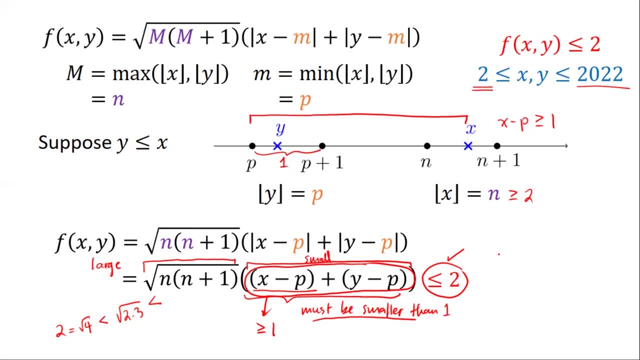 and f is less than or equal to 2,. this is now impossible. Okay, now impossible. Okay. so what was the assumption here? We were assuming here that x and y belong to two different intervals, And we saw that if x and y were to belong to two different intervals, f of x, y 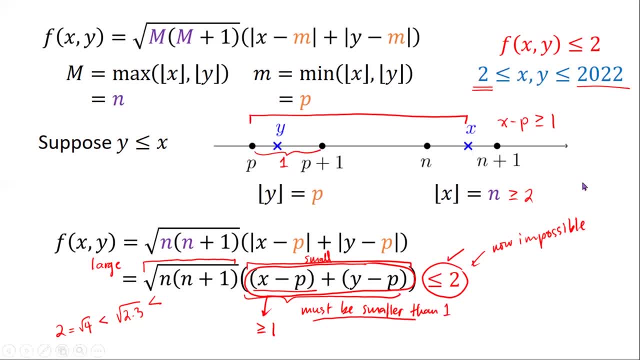 we cannot make it less than or equal to 2. That's impossible. We are forced to this conclusion that x and y must be in the same interval. They cannot be far apart for them to belong to different intervals. They must be in the same. 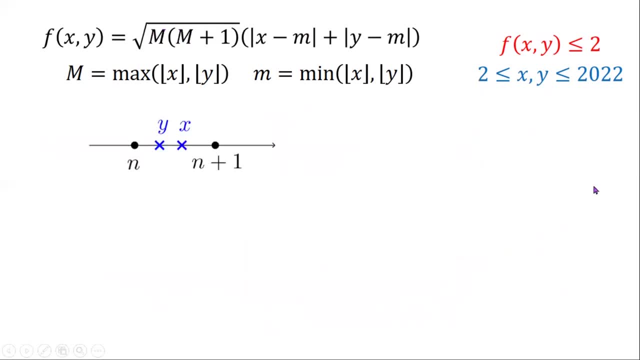 interval. All right. So now let's say x and y are between n and n plus 1.. So while x and y may not be equal, at least their floor function values are both n. So big M and small n Are both going to be n And you can infuse that into the function. All right, And then again, 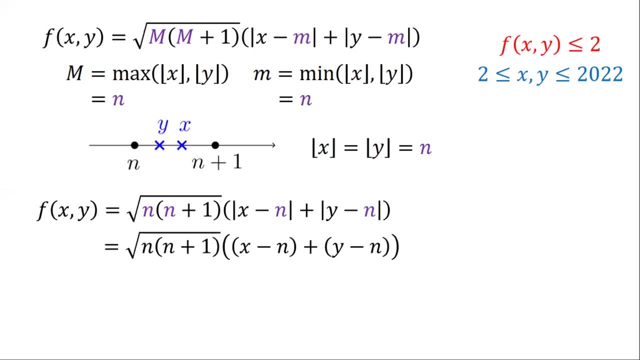 just like before, x and y are greater than or equal to n, So you can drop the absolute value bars And, in fact, the second factor. I will write that as x plus y minus 2n. So the condition that we want imposed now is that this should be less than or equal to 2.. All right, So this is what 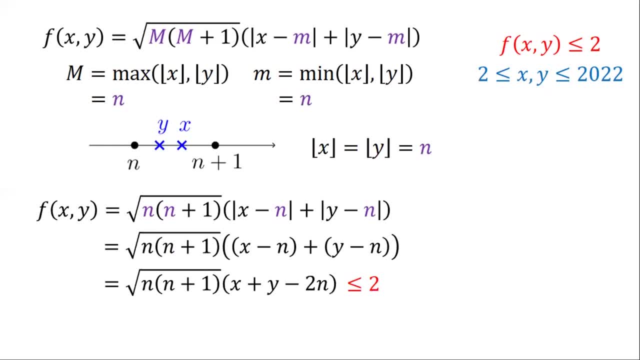 we need to happen. So x plus y minus 2n. So this is what we need to happen. So x plus y minus 2n Times that radical should be less than or equal to 2. Or in other words, x plus y should be less. 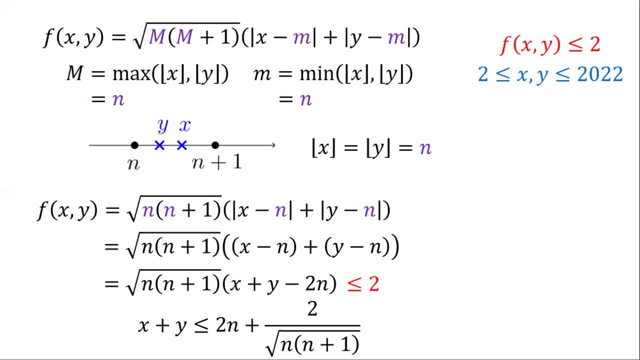 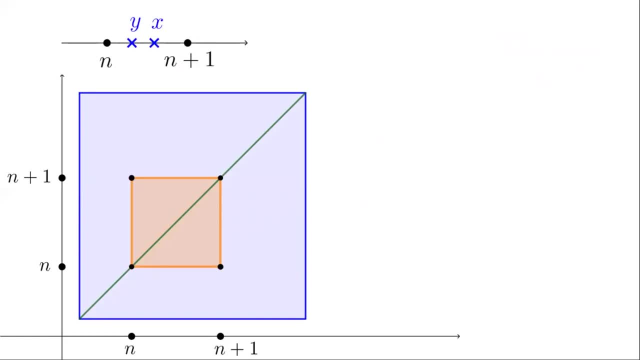 or equal to 2n plus that fraction. Okay, Now we're running out of space, So let's restart here. So all right. So let's say x and y, And they're in the same interval. Let's say from n going to. 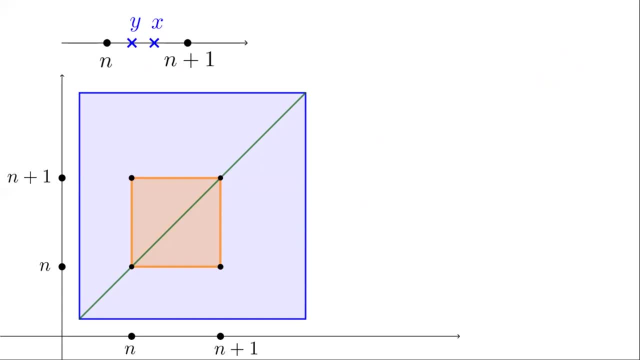 n plus 1.. So let's go back to the original domain, the blue square, And identified there on the x and y axes are the intervals from n to n plus 1.. So therefore, if you look at that particular brown square, this would be the collection of all points: x, y. 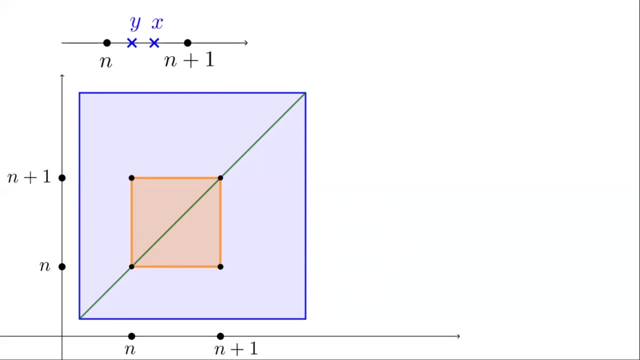 whose coordinates both of them are between n and n plus 1.. So now let's focus our attention on the points within this square for which the function value will be less than or equal to 2.. But we already Pointed out that it means this inequality must be satisfied by the x and y coordinates. 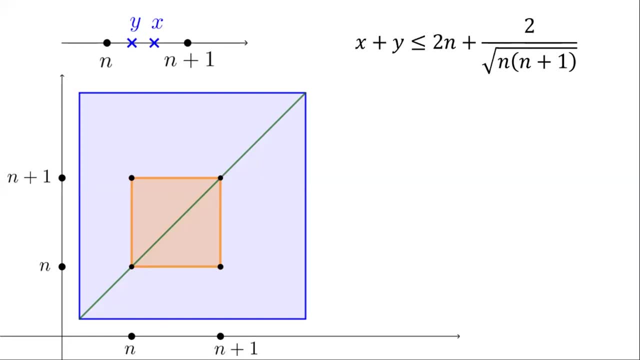 Now, this set of points x, y would therefore be a region below a line, And that line has equation x plus y equals 2n plus that fraction. So let's try to see within that brown square what are the points below this line. 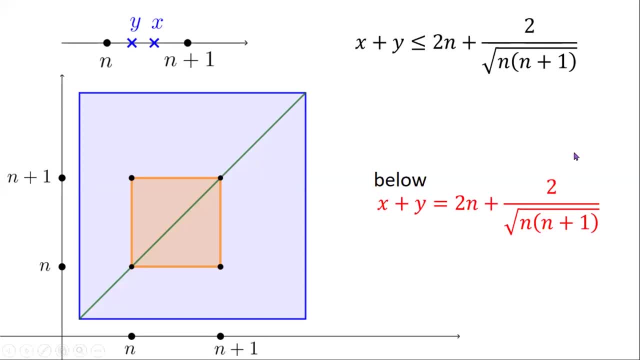 So first let's draw The line by selecting two points: y is equal to n, then x should be equal to that n plus 2 over the square root of n times n plus 1.. All right, So how do we know that red point is? 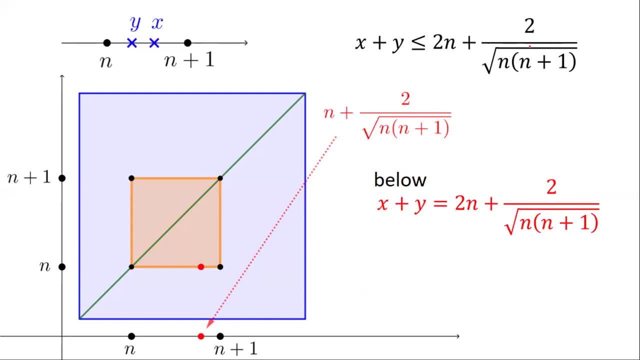 between n and n plus 1?? Because- remember this radical- we argued that this is strictly greater than 2, which means this fraction here, this is strictly less than 1.. So that red point would not be able to go beyond n plus 1.. 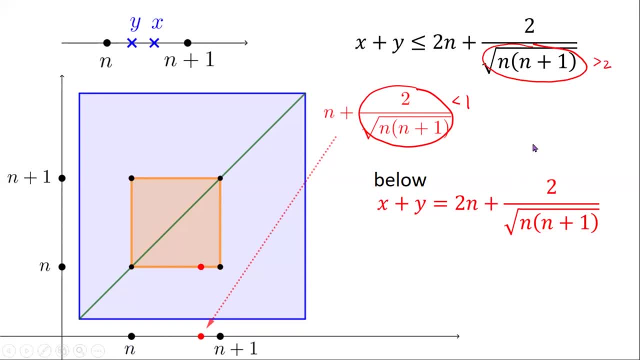 And the next: what if this time x is equal to n? So we're looking at the right vertical side of the square- then y should be n plus 2 over the square root of n, n plus 1.. So then, if you connect those, 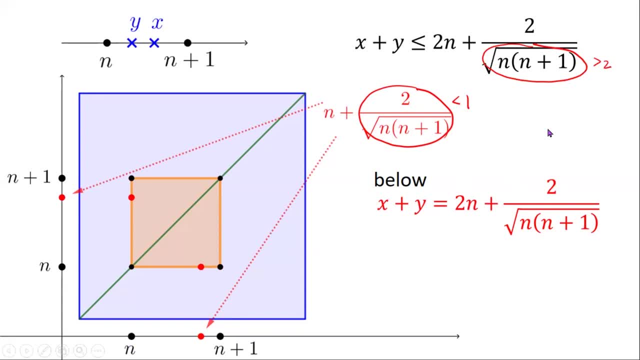 two red points on the bottom and left side of that brown square. you get the hypotenuse that would be part of the line. So that red point is the line that we have identified, And so the region below, which is inside that square, is that particular red triangle. So all points- x, y, whose coordinates are both between: 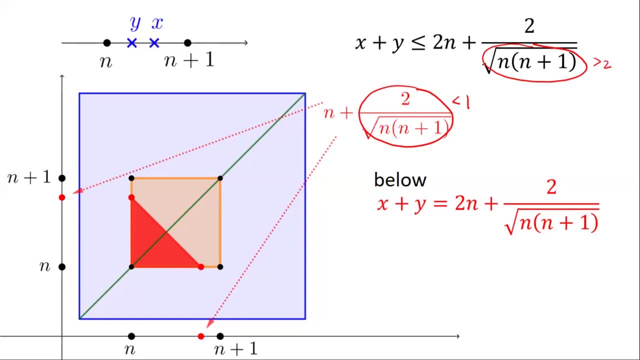 n and n plus 1, for which the function value is less than or equal to 2, are then precisely the points inside that red triangle, And so we are interested in the area of such a region. So it's here, And you can see that the section here has a little red line, And so we want to multiply that. 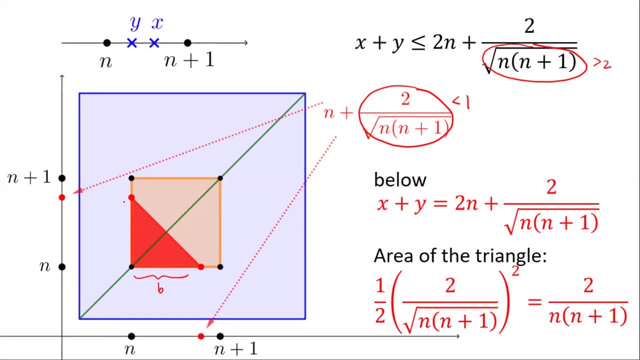 by 2 over the square root of n times the base and height. So the base is this and the height is equal to the base, And that base is this: this fraction: 2 over the square root of n times n plus 1.. So you square that, multiply it by 1 half. You get 2 over n times n plus 1.. This is now the area. 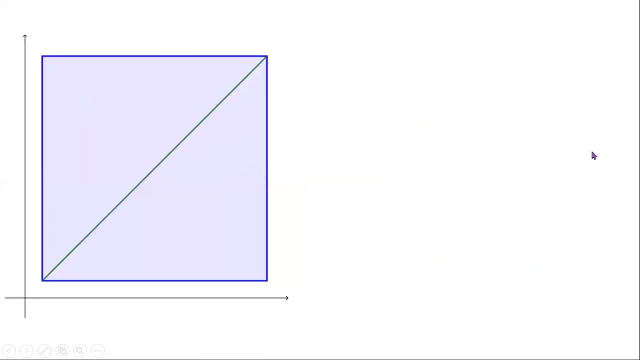 of that red region. So back to the original problem. we want f of x, y to be less than or equal to 2.. and we identified how, if x is between n and n plus 1, so with y, then the set of points x, y. 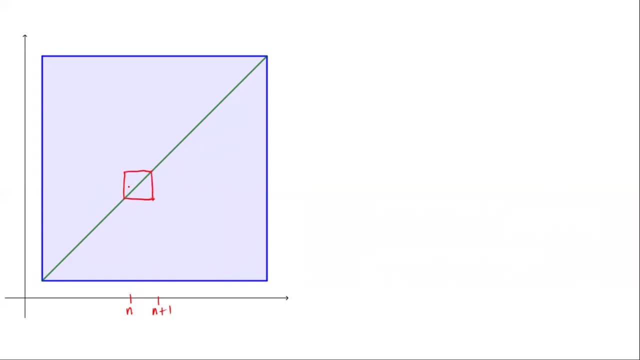 satisfying the inequality that f is less or equal to 2 would be points on a red triangle such as this, And this observation applies to other intervals, such as the very first one, the interval from 2 to 3, so corresponding to the case where n is equal to 2.. So we are looking at 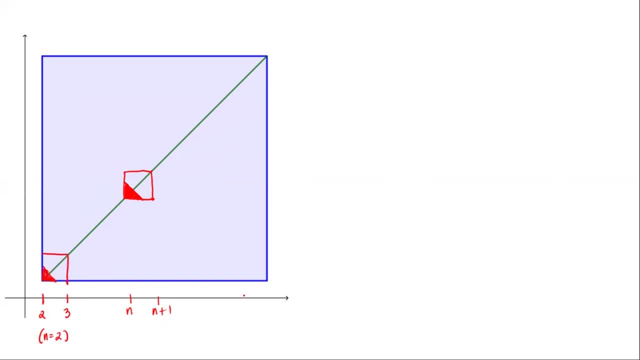 a triangle like this and up to the very last interval, from 2021 up to 2022.. So that's for the case when n is 2021.. We are also looking at a triangle like this. Okay, So the red triangles. 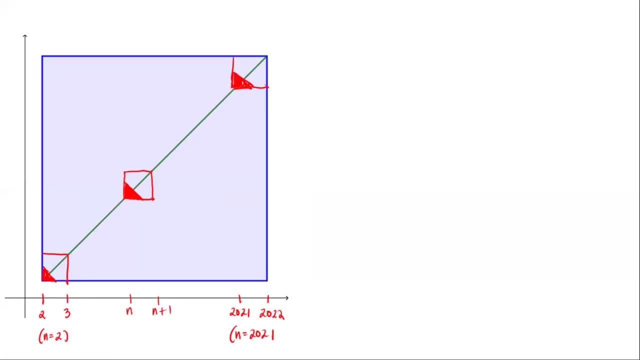 that we have here are the ones that we are looking at. So we have a triangle like this. So we have a triangle like this. So we have a triangle like this. Okay, So the right triangle is we want they have different sizes. all right, but of course my hair up. now you're doing silly d. 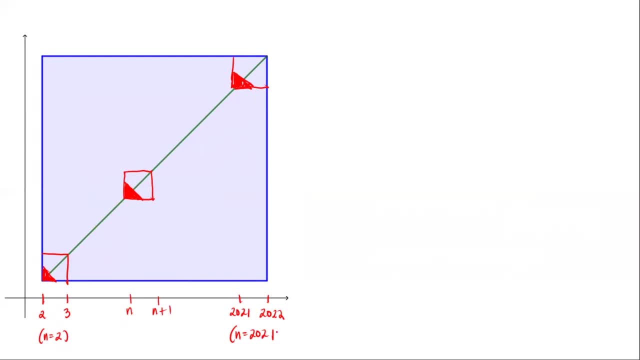 there's such that different sizes, but uh for values, values of n, the area is uh two over n times n plus one. so that's how they're going to look like. so if you draw somewhere of those red triangles, so going to number points x, y, such that f of x, y is less than or equal to two, so too many. 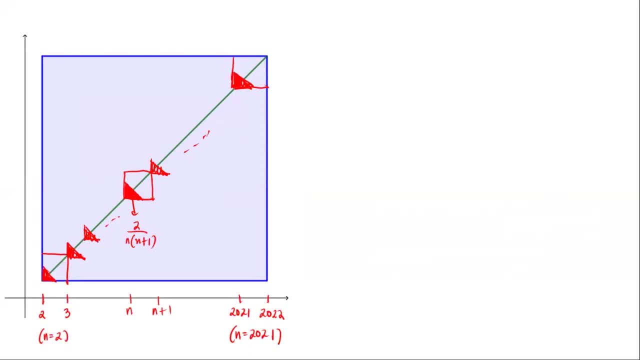 to draw. so i'll just put dot, dot, dots. and the areas are given by two over n times n, plus one where n runs from two, three onwards until 2021. so this summation s, this is now the sum of the areas that we are looking for all right now. this is an example of a telescoping series. 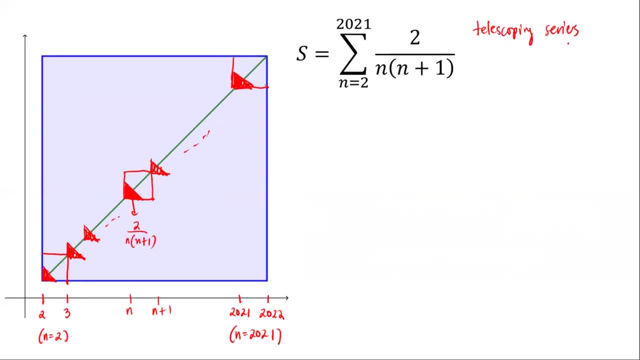 so, in case you are not familiar, i have an addendum to this video. so at the end, where i talk briefly about telescoping series, but for those who have recognized that this is a telescoping series, uh, we are able to exploit the fact that each of these terms two over n times. 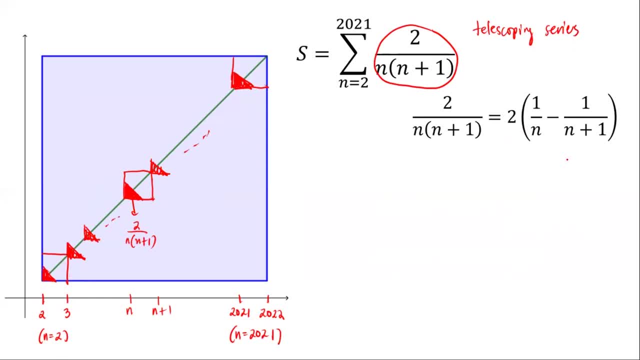 n plus one can actually be written as a difference: double one over n minus one over n plus one. this is a fact that you can verify by algebra, for the unfamiliar might hear a easy pen. but anyway, let's see here. there is a difference between two half and one-third, so you get one-third. 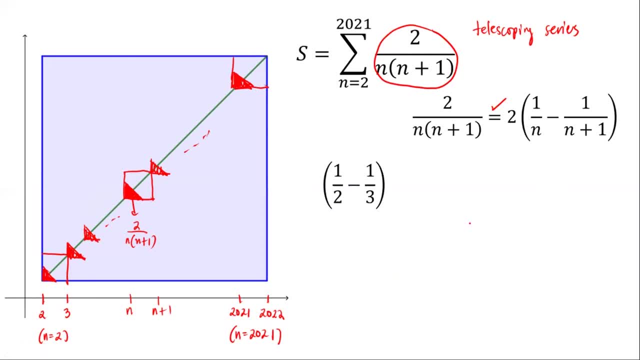 okay, so, uh, from the other side, this is a Dirac's formula- the difference between two half and one third is one-third, which in the formula is typically about one-third. it's one-third. so when you're assuming it's true, well then, how does that help us all? right, because, uh, 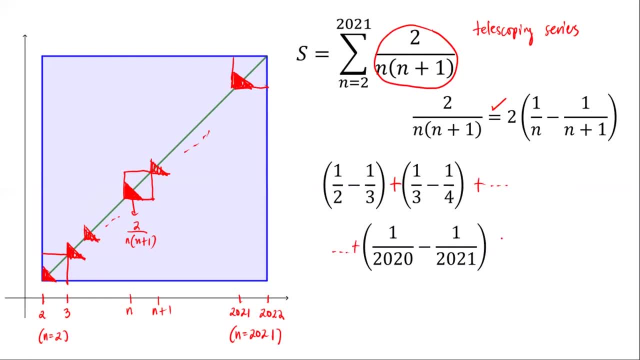 the difference is one over n minus one over n plus one when n is equal to two. so you get one-half minus one-third, and then, when n is equal to three, you get that difference and then uh, you get uh 2021. but of course, do not forget that this is going to be doubled, multiplied by two, because 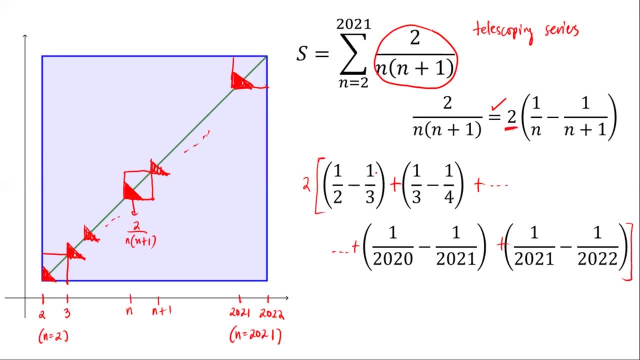 of this factor here. now, even though there are so many fractions, we observe that, fortunately, a lot of them are going to cancel each other out, leaving us with just one half and one over 2022 that we need to subtract, which we need to double, and the computation is now relatively easy, and 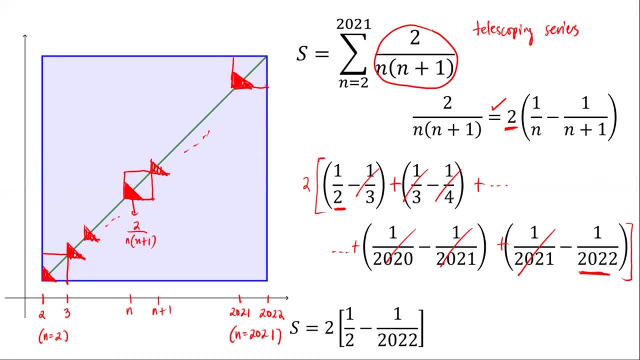 straightforward, of course, after recognizing we have a telescoping series, so this is what we get. this is the sum of the areas 1010 over 1011, which means, with this as a and b, the answer that we are looking for a plus b is equal to two zero. 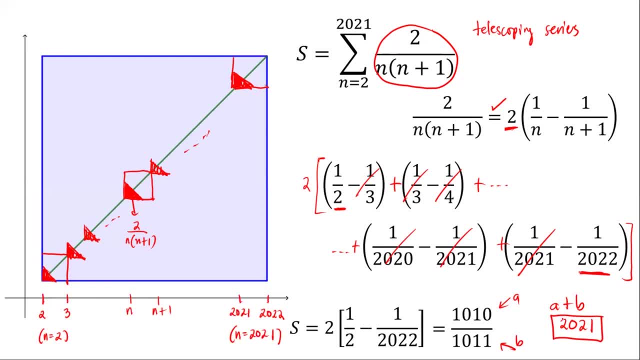 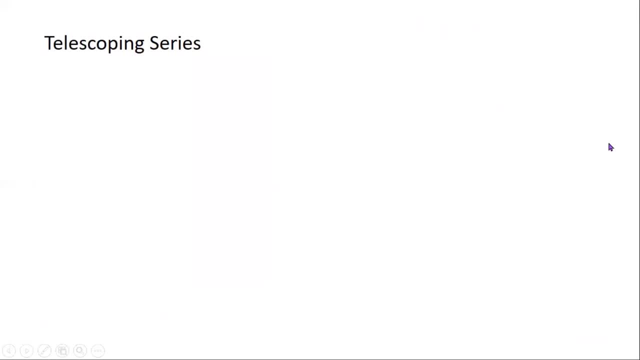 to one. this is the answer to problem number 25.. yay, okay, for those who are not so familiar with telescoping series. so here's an example. let's find the sum, as n runs from 1 to 20, of 5 over n times n plus 2.. so what happened earlier? in the main part of the solution was: we saw how 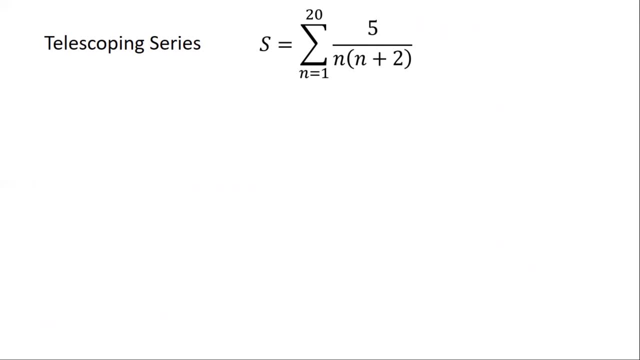 similarly, the denominator is the product of two linear factors and then the numerator is a constant. similarly, we can rewrite each of these terms as a difference. so the task now is to figure out how is that difference going to look like? well, we look at two fractions with denominators n and n plus 2, so let's look at this. 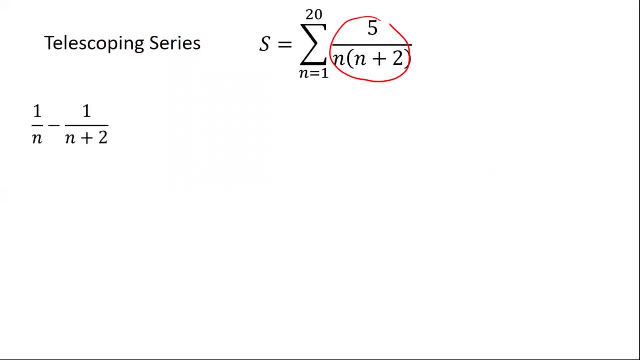 difference 1 over n, first, followed by 1 over n plus 2, so that the difference is going to be positive because the terms of the series are positive. and then you can verify that this is going to be 2 over n times n plus 2. well, in the series the numerator is 5.. so we just multiply this by 5 and then divide. 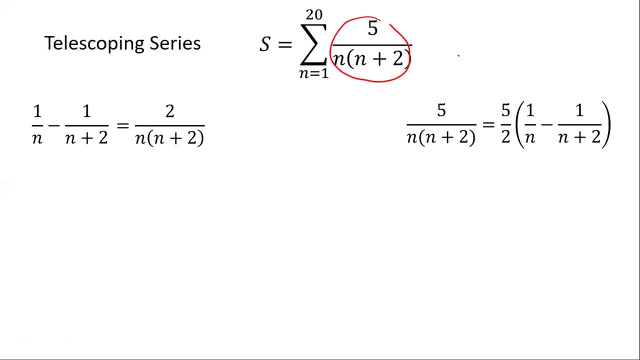 by 2, so that means the terms 5 over n times n plus 2, that's equal to 5 halves of differences: 1 over n minus 1 over n plus 2.. so now when we evaluate the series- sorry, that's supposed to be up to 20.. so here, 20.. so instead of adding 20, 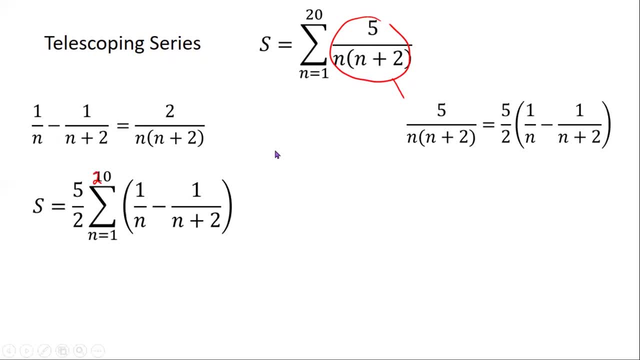 fractions. let's write each term as a difference. so these are some of what we're going to see. so before the five halves. all right, five halves. so, when n is one one minus one third, this is what you get when n is equal to two and when n is equal to three, and then 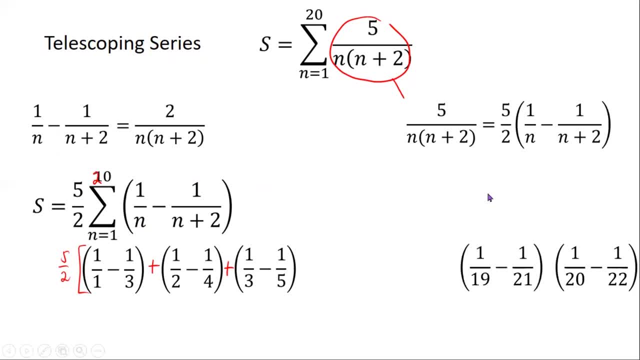 lots to right here. so that's the very last, and then, uh, the terms just before it all right. and then we see that one minus one third, and then when you go to one half minus one fourth, nothing cancels yet. but when you get to the third group, finally minus one third, plus one. 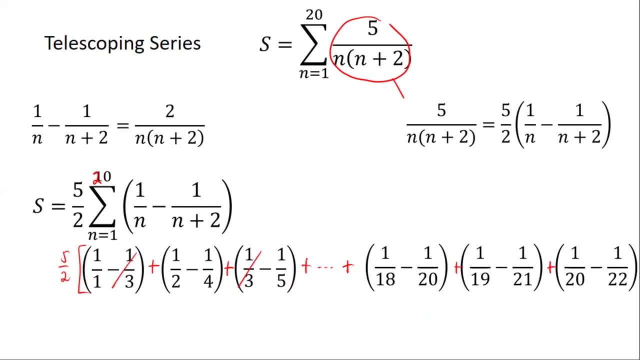 third. and then we see that, uh, although i it's not written here- minus one fourth will be cancelled. and coming from the right side, we see minus one over twenty plus one over twenty cancelling each other. so it follows that one over nineteen is also going to disappear. so the only thing surviving are 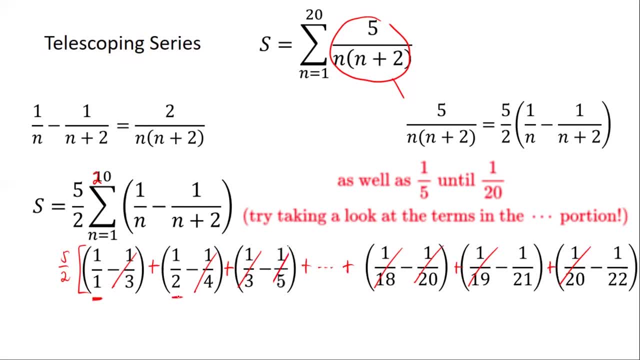 these um fractions whose denominators are one and two. but when the denominator starts from three and then four and then from the other side, if the denominator is 20 and then lower like 19 or 18, it's going to disappear, but when the denominator is 21 or 22, it's going to stay. so that means the sum is equal to five halves. 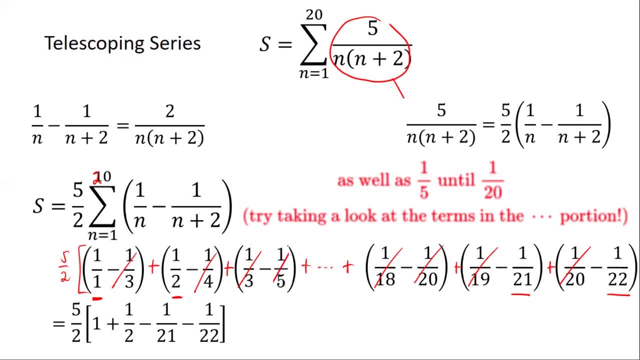 times this sum and difference of four fractions. definitely so much better than uh, than doing the operation on 20 fractions, so i will not compute this anymore, because i just wanted to illustrate telescoping series. so all right now, of course. uh, the time it took to explain this solution. 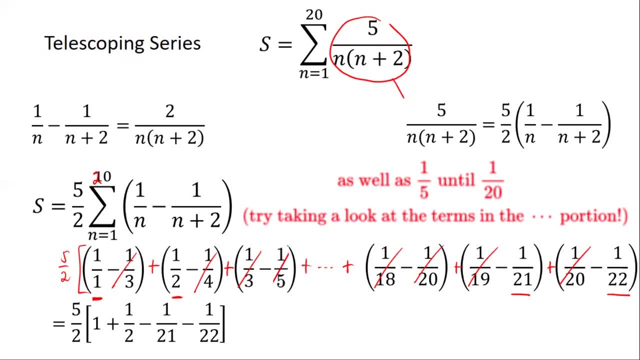 is longer than um, i suppose what would be possible or feasible within the philippine mathematical olympians. so, especially when you get to the latter parts, you may not be able to solve them within the time that's provided. it requires a particular kind of skill set. but even if we cannot solve,